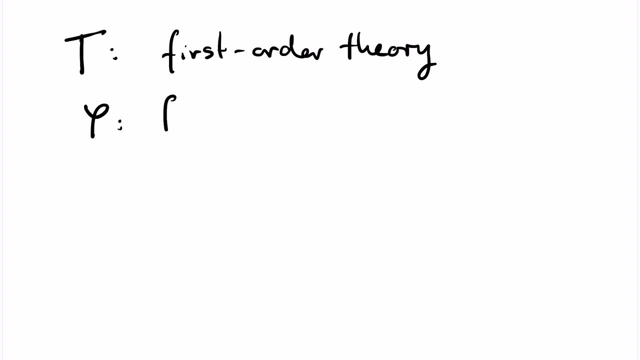 fixed first-order theory, t, and where we would like to know whether t implies some first-order sentence, phi, For example, if t is the theory ZFC and phi is the well-ordering theorem, then the answer would be yes. Or, as another example, we might want to know whether ZF. 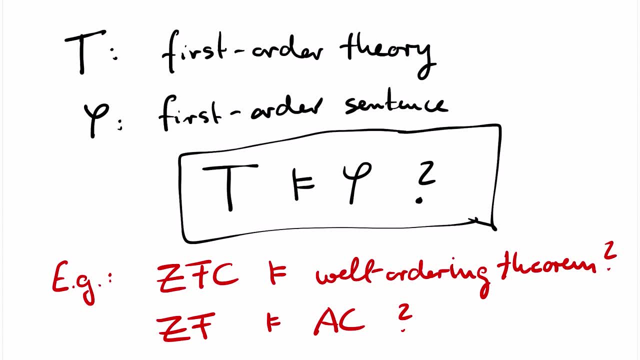 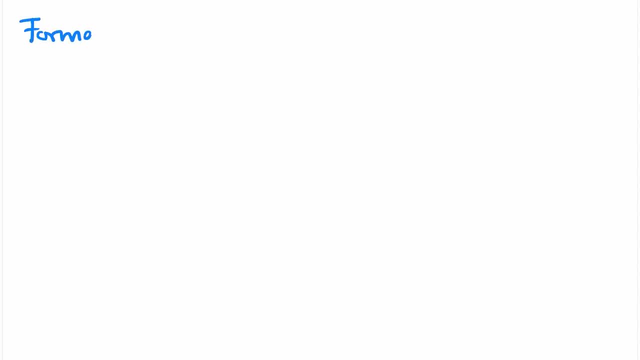 implies the axiom of choice. just as an example, You can replace the axiom of choice by any mathematical statement that you are interested in. A formal proof in t is simply a finite sequence of sentences. Each sentence in this sequence is either a logical axiom- these are first-order sentences that hold in all structures- or a. 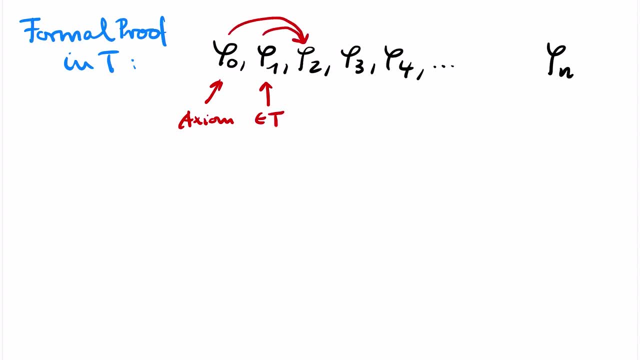 sentence from t Or it can be derived from two sentences that come earlier in the sequence by a simple proof rule. This is called modus ponens. We already know modus ponens from propositional logic. It states that if phi is a tautology and phi implies psi is a tautology, then psi is a. 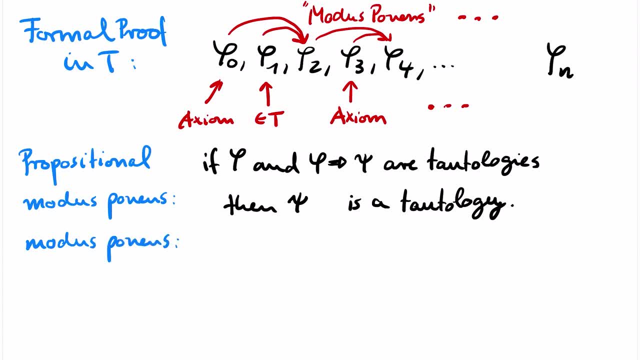 tautology There is the following variant of modus ponens for first-order logic: If t implies for all x phi and t implies for all x phi implies psi, then t implies for all x psi. So if phi 0 and phi 1 are sentences in my proof that look as in the assumptions of modus. 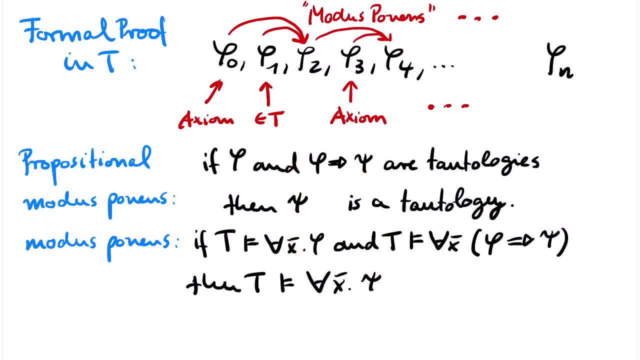 ponens, then phi 2 may look as a sentence. in the conclusion of modus ponens We write t vert-phi and say that phi has a proof in t. If there exists a formal proof in t, that ends with phi. 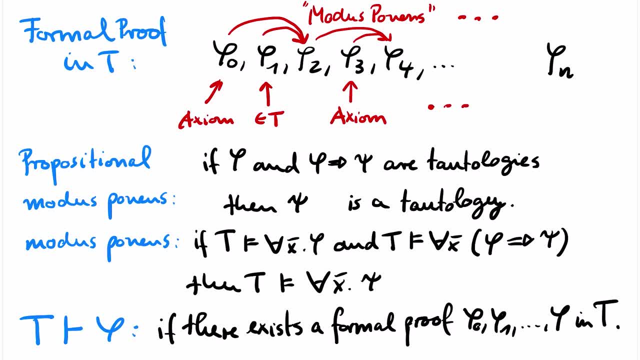 All that remains for introducing my formal proof system is to specify what the logic is for the first-order logic. That is, if the first-order logic is the final product of the first-order logic, then I need to specify what the logical logic for the second-order logic is. 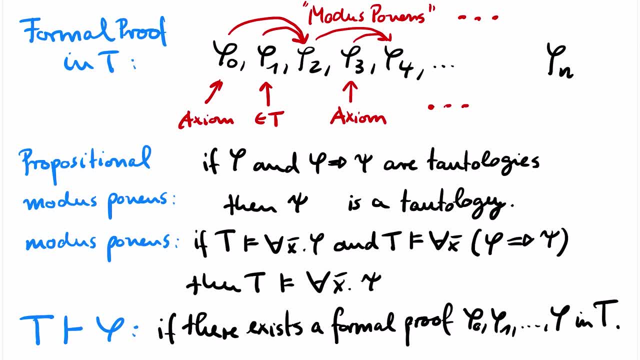 And, by the way, you can also specify what the logical logic for the first-order logic is. for the first-order logic is, axioms are that we can use in our formal proofs. I start with axioms about fundamental properties of the equality relation. 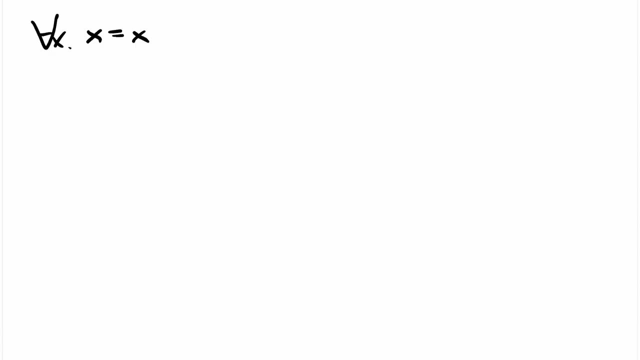 The first axiom is for all x: x equals x. This is called E1 and it expresses that equality is reflexive. The second axiom is for all x and y. x equals y implies y equals x. This is called E2 and expresses that equality is symmetric. 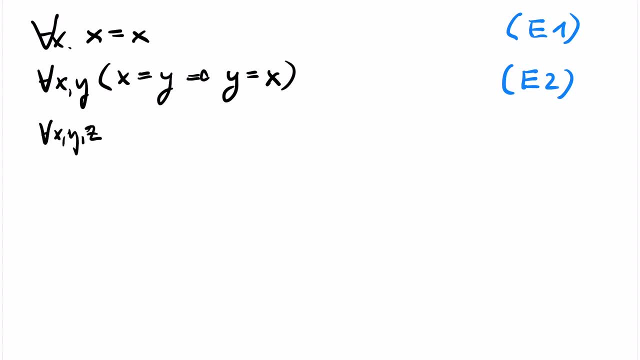 The third axiom is for all x, y and z. if x equals y and y equals z, then x equals z. This is called E3 and expresses that equality is transitive. Then I need for every function symbol f of arity, n in the signature. the axiom. 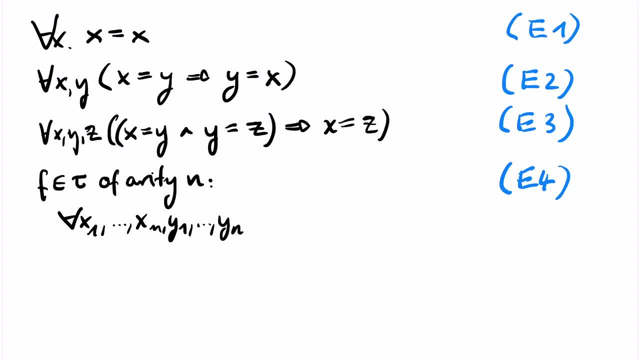 for all, x1 up to xn and y1 up to yn. if xi equals yi for all, i then f applied to x1 up to xn equals f applied to y1 up to yn. This is called E4 and it states that equal things behave. 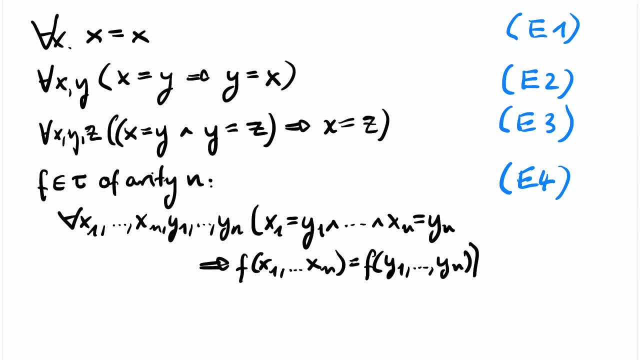 equally under function application. We have a similar axiom, E5 for equality with respect to relation symbols instead of function symbols. So we see that the set of axioms, and therefore also our proof system, depends on the signature. It should be clear that all of these sentences 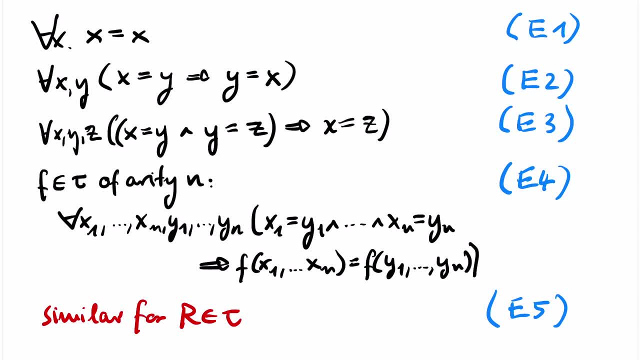 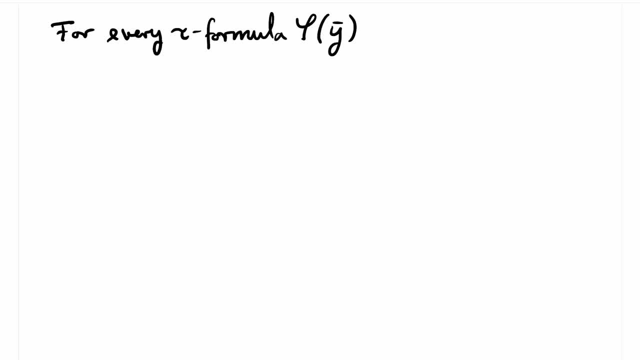 hold in all tau structures. The next axiom is actually not one axiom, but infinitely many. For every first total tau formula phi with three variables y and for every variable x, we have the axiom for all y phi implies for all y and for all x phi. 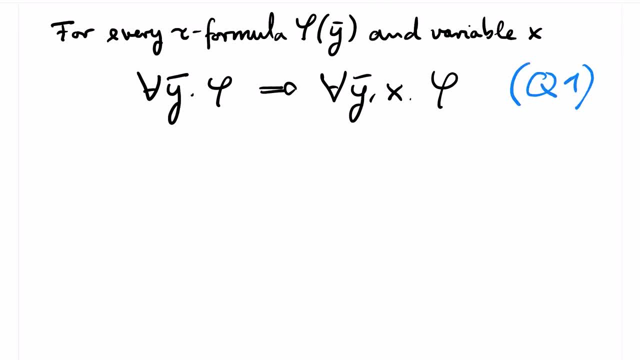 This is called Q1.. The Q indicates that it is an axiom about quantifiers. Clearly this sentence holds for all tau structures On the right. we just added a dummy variable which has no effect on the truth value of the sentence. I will present two concrete instances of Q1.. 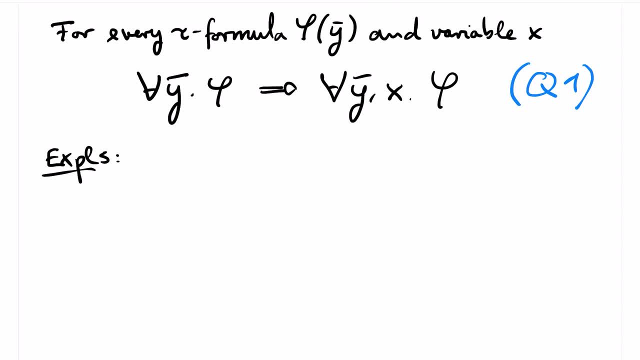 For the signature that just contains a single unary relation symbol, r. The first is for all z- r implies for all z and x r. So here we instantiate phi with the formula r. The second example is: for all z- r implies for all x, for all z. 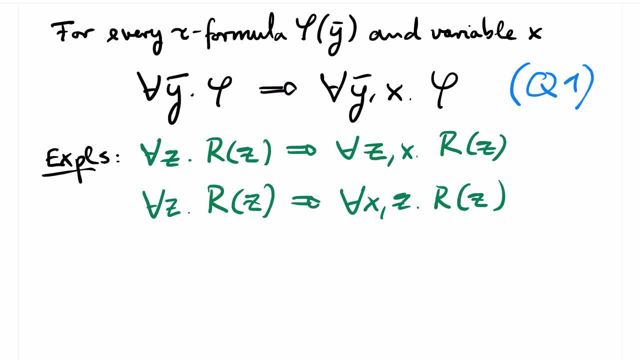 r. Note that here the order of the variables x and z is flipped. The reason is, that here we instantiated phi with the sentence for all z, r, And the universally quantified string of variables y in Q1 is empty. Also, Q2 consists of infinitely many axioms. 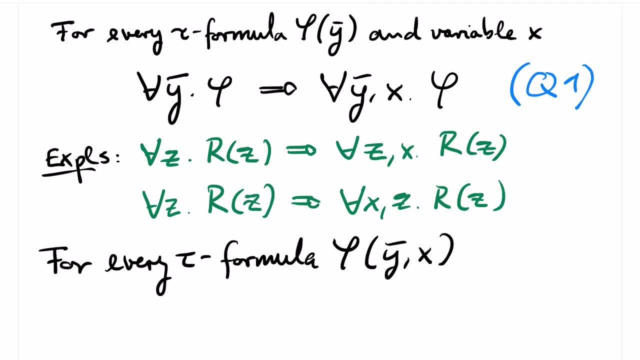 We have for every tau formula phi, with three variables y and three variables x, the axiom that says for all y, if for all x not phi, then there is no x, such that phi. It is clear that also Q2 holds in all tau structures. 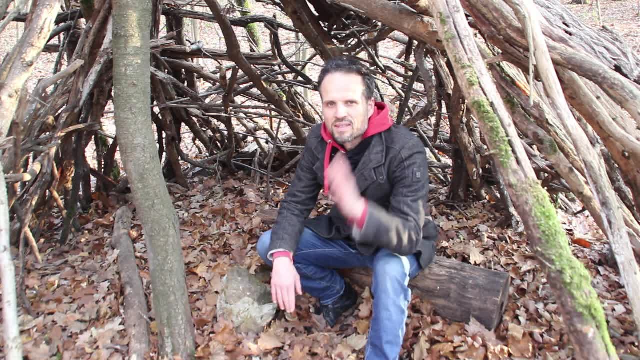 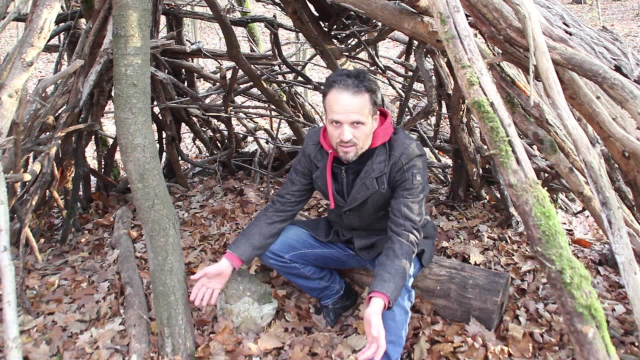 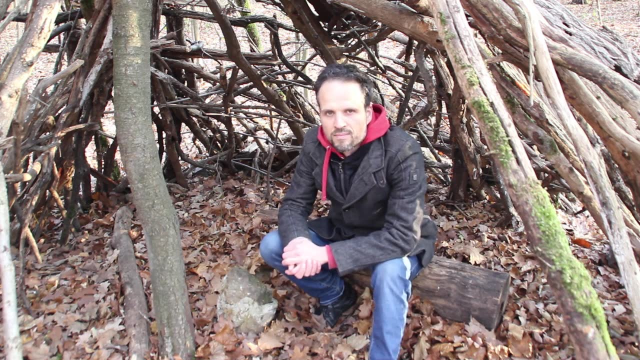 Infinitely many axioms, You might say: stop, this is cheating. If you allow infinitely many axioms, you could simply allow all valid sentences as axioms And that would give you a sound and complete proof system. So that's cheating. And that brings me to a very 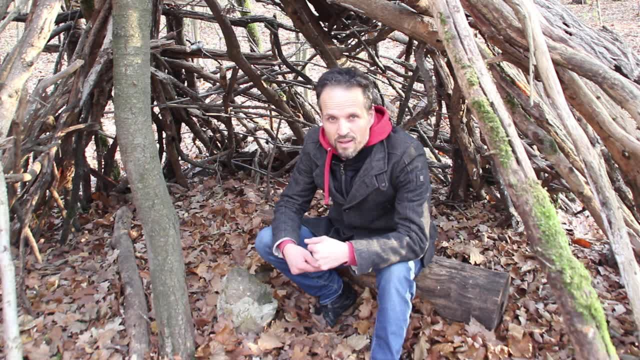 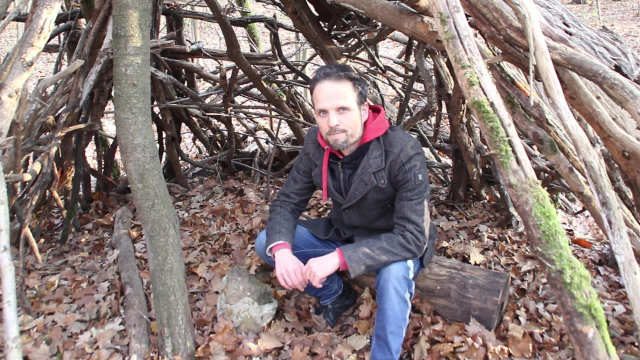 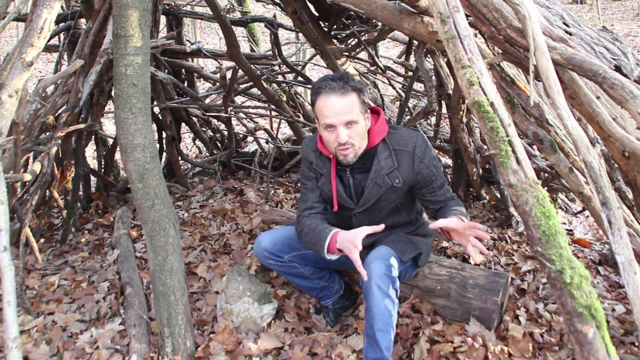 important feature of our proof system. Our proofs can be checked by a computer, Even in polynomial time. So all the axioms that we have seen so far. it is so easy to check from a given first order sentence whether it is one of those axioms. 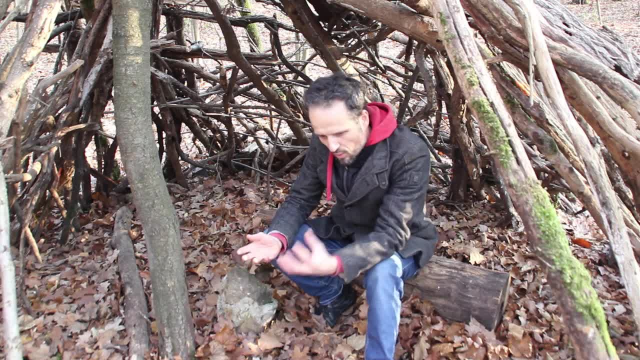 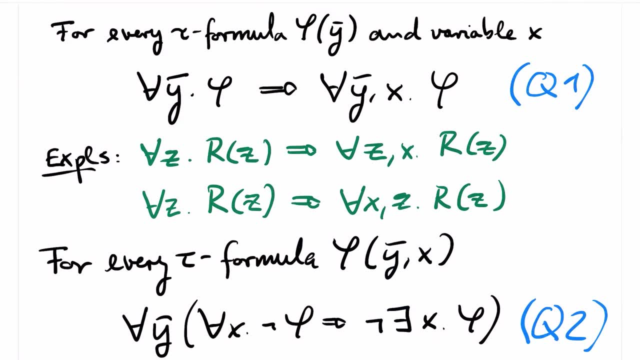 And it is also easy to check whether modus ponens is applied correctly. The axioms that we have introduced so far can be checked by a computer. For Q1, we simply have to decide whether there exists a formula phi such that the sentence is of the given form. 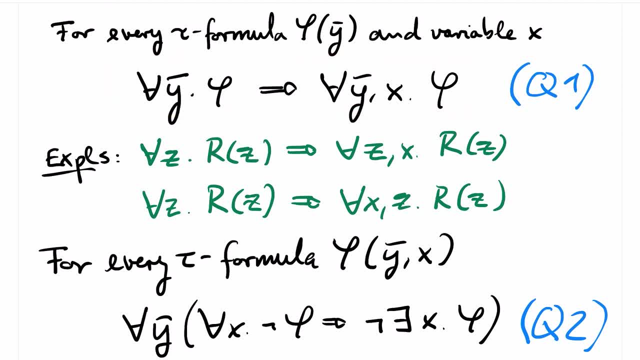 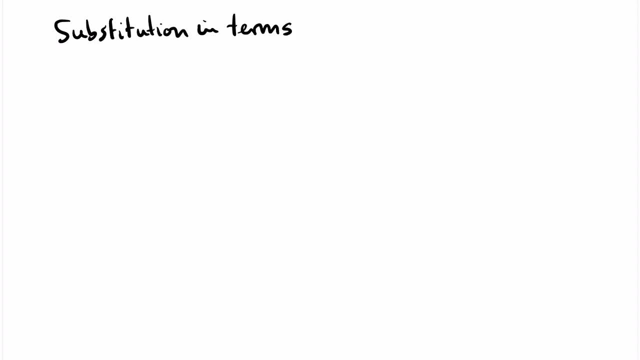 It is easy to write a computer program to do that. There is no brain required for doing that. To specify the next axiom, we need the concept of substitution. Let s and t be tau terms and let x be a variable. We write s square brackets: x maps to t. 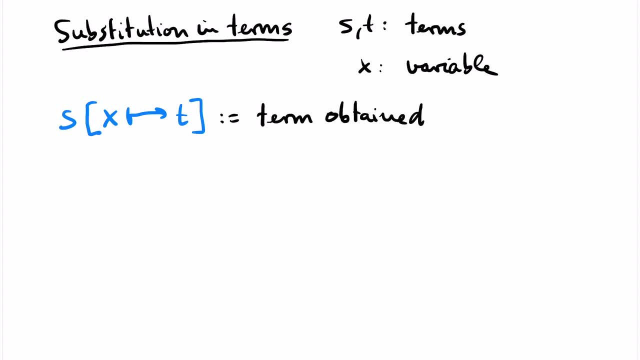 for the term obtained from s by replacing all three occurrences of x by t. So, for example, if we have f square brackets, x maps to g of g of y, then we will obtain the term f of g of g of y, comma y. For this notation there are: 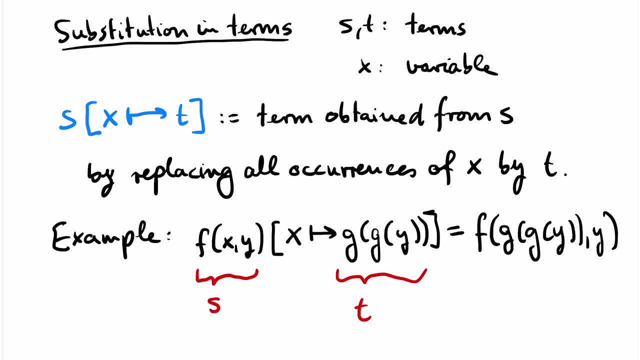 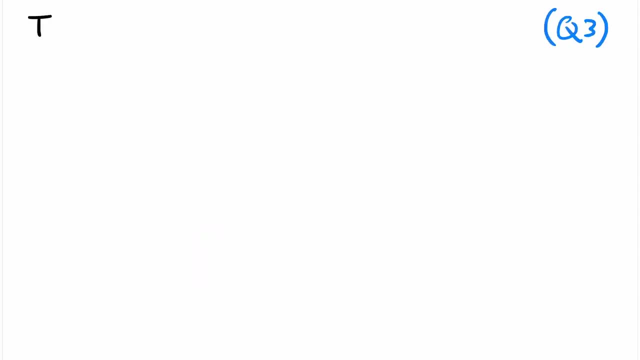 many, many variations in the literature. Almost every author has her own convention, so I picked the notation that I found most intuitive and has less clashes with other notation in the course notes. Axiom scheme Q3 has, for every tau formula phi with three variables. 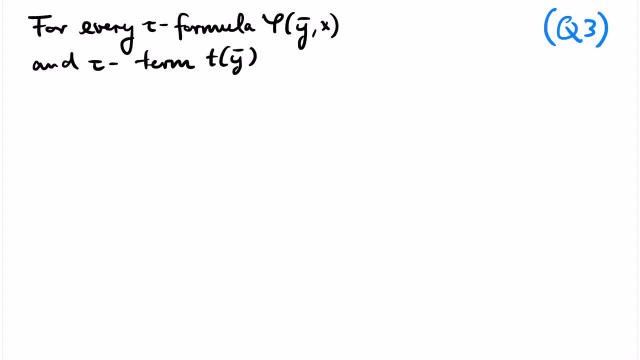 y and x and t, a tau term with variables y and t. The sentence for all y phi- replace x by t- implies there exists an x phi. Again, it is clear that this sentence holds in all tau structures simply because the term evaluated for some values in the structure. 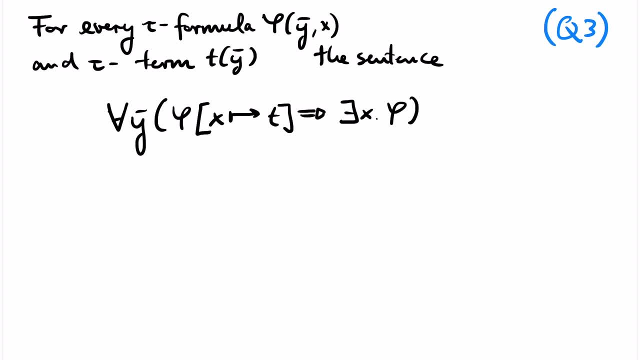 provides a witness for the existentially quantified variable x. The next axioms are formed by the formulas phi and psi, with three variables: y and the variable x. that is not free in phi. We then have the axiom for all y, for all x. phi implies psi. 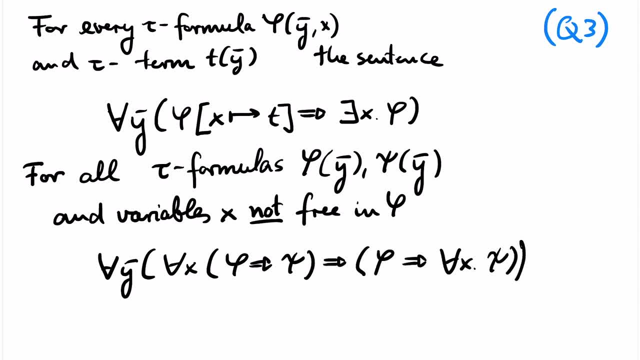 implies phi, implies for all x psi. This is axiom Q4 and Q5 is just a converse. If you have a converse, look at these sentences, then you see that they hold in all tau structures again. Finally, we have the axiom scheme taut for 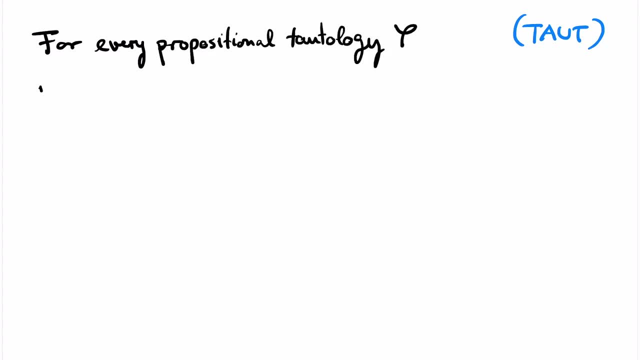 tautology For every propositional tautology, phi, with propositional variables x1 up to xm and for all first order tau formulas psi1 up to psim. with three variables x, we have the axiom for all x phi of psi1 up to psim. 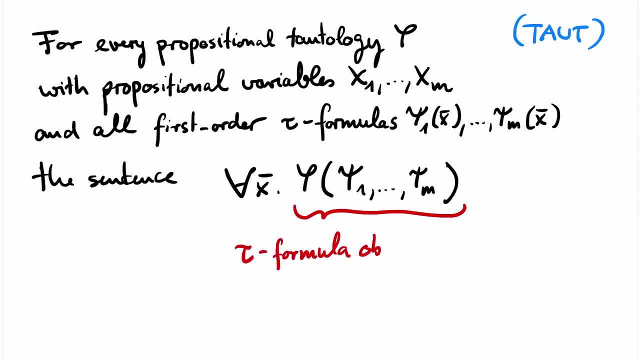 Where phi of psi1 up to psim denotes the formula obtained from phi by replacing each propositional variable xi by psii. Again, it is clear that since phi is a propositional tautology, the resulting sentence is valid. Recall that we have seen. 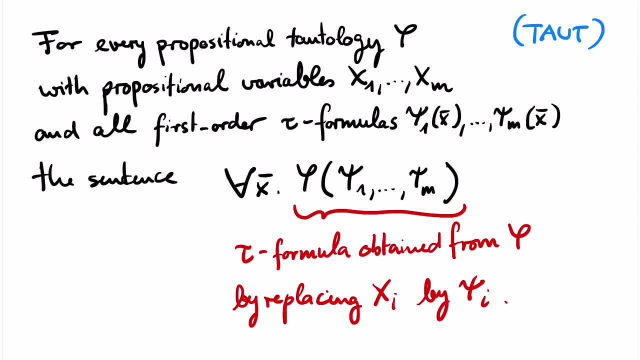 several algorithms in an earlier video about the satisfiability problem for testing whether a given propositional formula is a tautology. It follows that the axioms from taut can also be checked by a computer. Instead of taut we could have used a smaller set of propositional 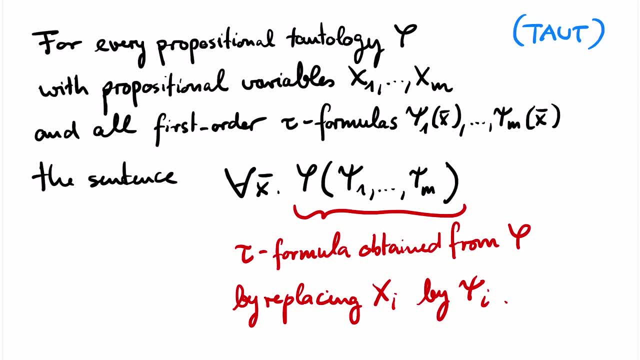 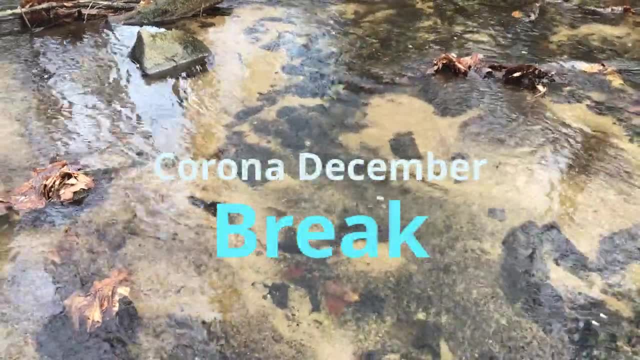 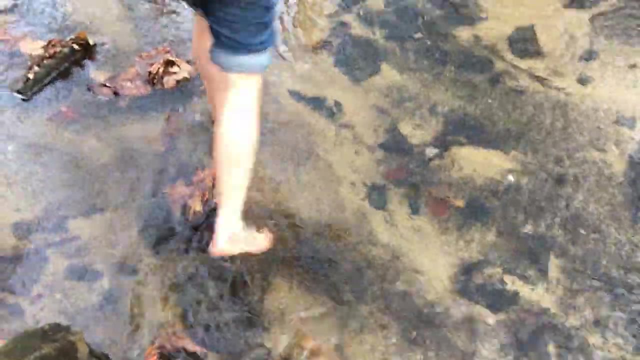 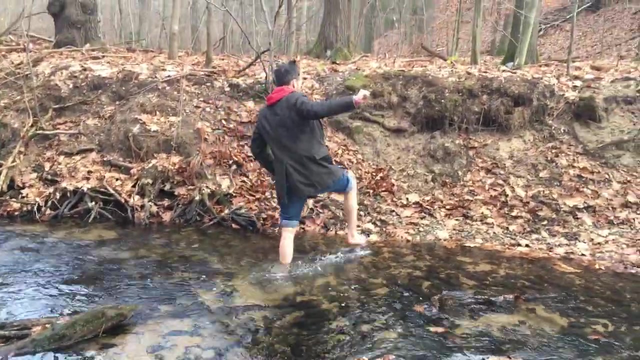 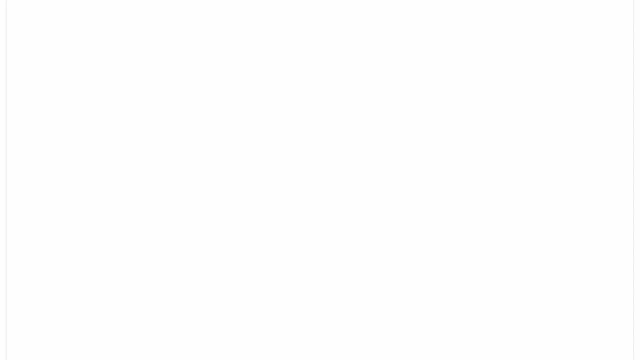 axioms that go back to Jensen, with the advantage that then we can even check in polynomial time whether a given sentence is an axiom or not. But to keep things simple, we will work with taut in this course. I will give an example of a. 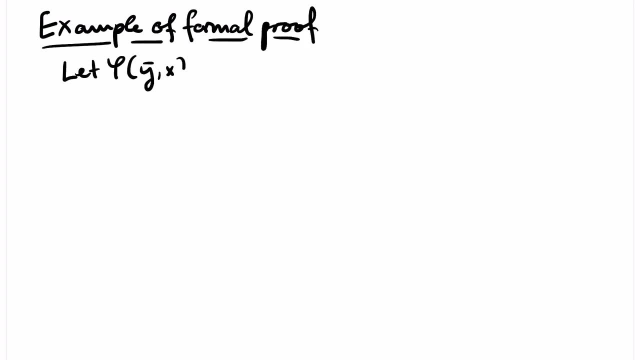 formal proof: Let phi be a tau formula with three variables, y and x, and let t be a tau term with variables y. Then, over the empty theory, there is a formal proof of the sentence: for all y, for all x, phi implies phi, where we replace x by the term. 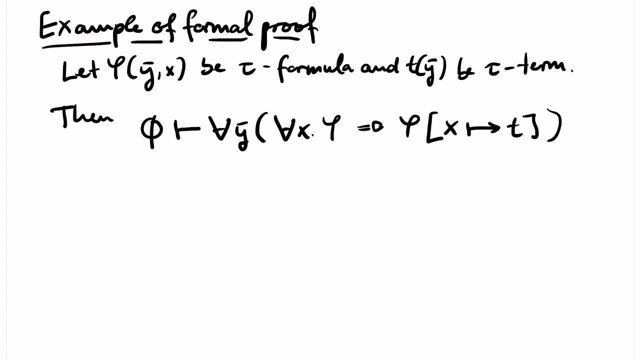 t. Semantically it is quite clear that this is a valid sentence, because if a statement holds for all x, it holds in particular for the value returned by t. But we want a formal proof of this statement. I warn you, these formal proofs are not easy to read. I will use 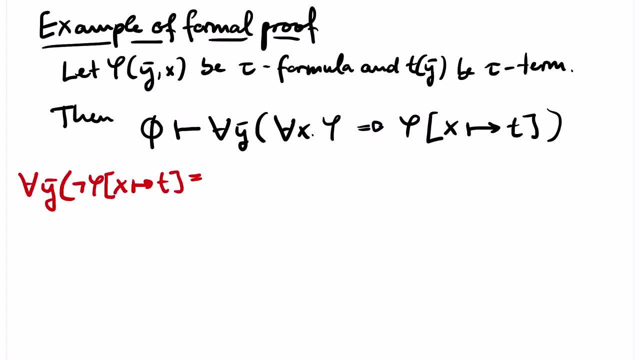 the axiom q3 for the formula not phi and the term t, which is for all y not phi, where we replace x by t, implies exists x not phi. Our next sentence in the formal proof is a bit long so that I don't read it out loud, but I just write it. 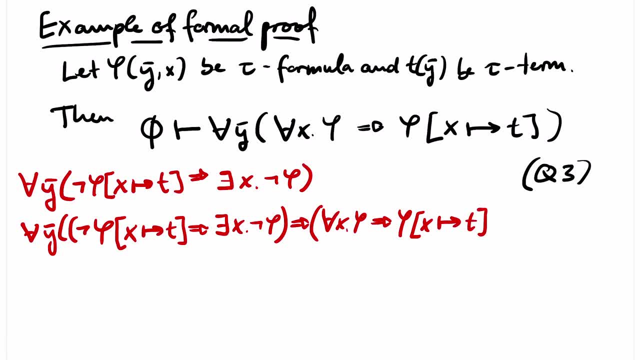 and explain it after writing. I claim that this sentence is an instance of taut Because it states the principle of contraposition: If not x implies y, then not y implies x. Our next sentence in the formal proof is the sentence that we want to prove. 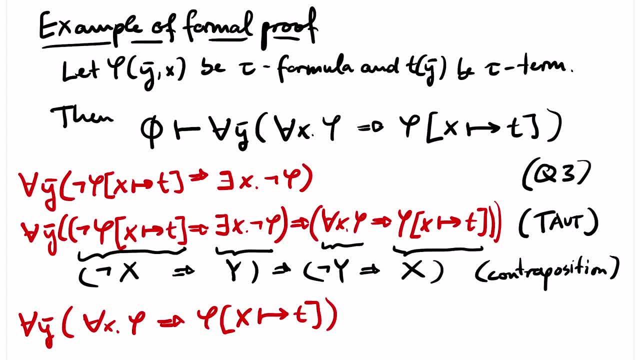 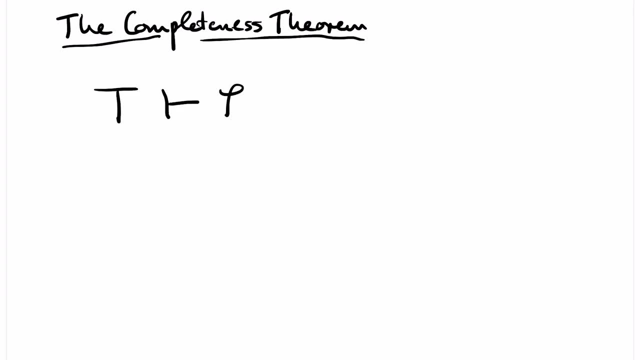 eventually, namely for all y, for all x. phi implies phi x replaced by t, And we obtain it by modus ponens from the previous two sentences. The completeness theorem takes the following short and elegant form: Phi has a formal proof in t if and. 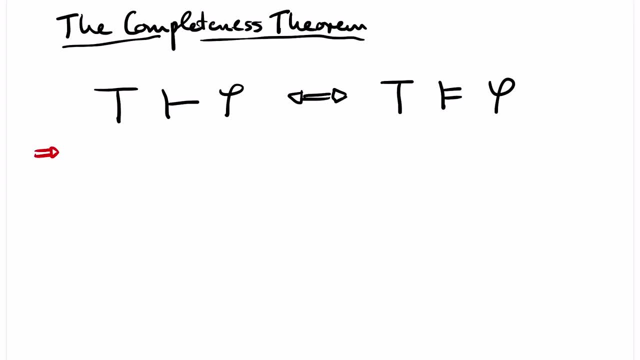 only if t implies phi. The forward direction in this theorem is easy to prove by induction over the length of the formal proof. For the converse, suppose that phi does not have a formal proof in t. We have to show that t union the negation. 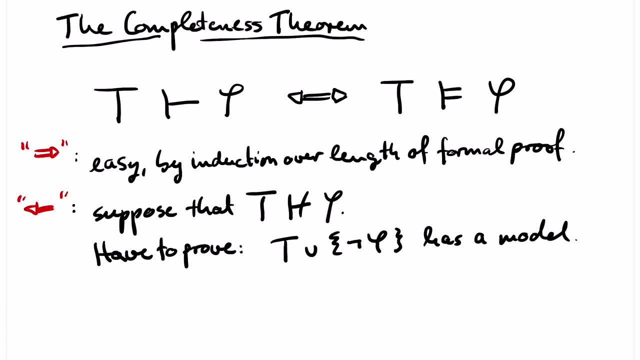 of phi has a model, So we have to construct a model, And the construction that we use is called Henking construction. The idea is to add new constant symbols. By new, I mean that these constant symbols are not in the signature of t and. 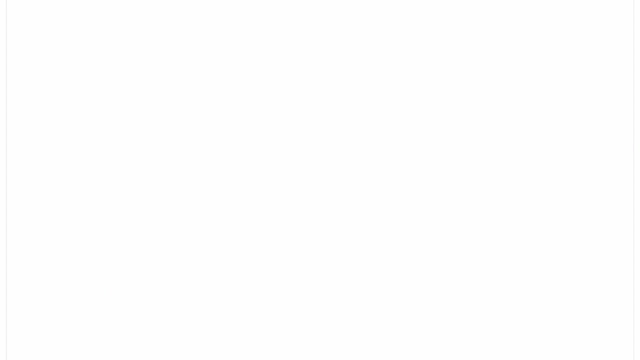 phi In the signature that we started with. A Henking theory is a tau union rho theory, such that for every tau union rho formula phi with free variable x, there exists a constant in rho such that the theory t contains the sentence: if there exists an x such that phi of x 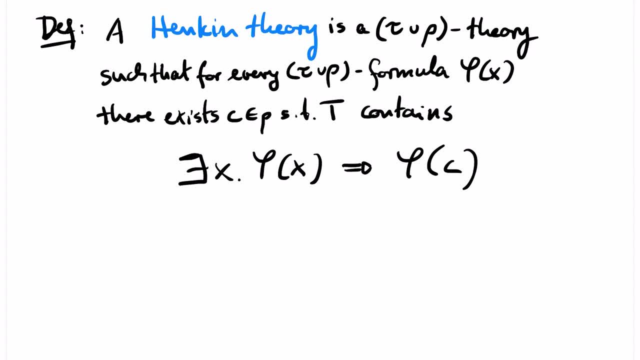 then phi of c. The constants from rho will then be called the Henking constants of t. Where do Henking theories come from? Well, if a is a tau union rho structure, such that every element of a is denoted by some constant from rho. 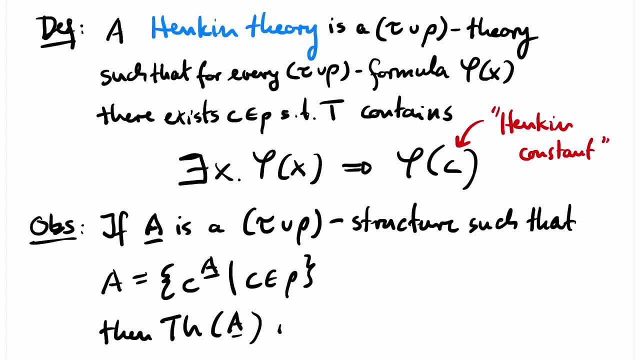 then the theory of a is a Henking theory. This is because if exists x, phi of x is true in a. there must be some element of a that satisfies phi, And there must also be a constant c in rho that denotes this element, And hence we have phi of c. 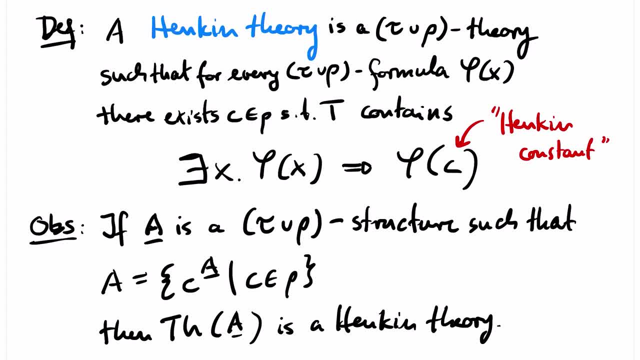 So the theory of a contains all the sentences that we need for Henking theories. Our first lemma will state that under a certain extra condition, there is a converse to this observation. For every Henking theory t that meets this condition, there is a structure a. 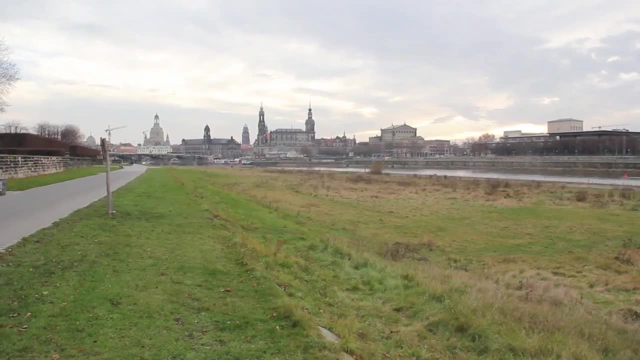 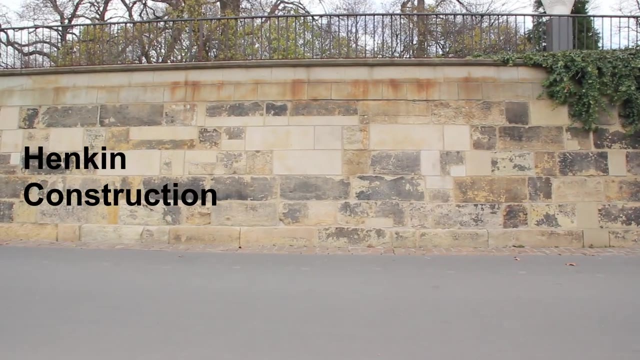 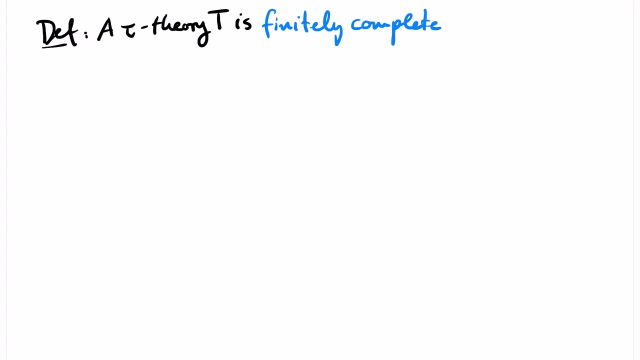 such that t is the theory of a, A tau theory. t is called finitely complete if first is consistent, That is, there is no tau sentence phi, such that there is a formal proof of phi in t and a formal proof of not phi in t. 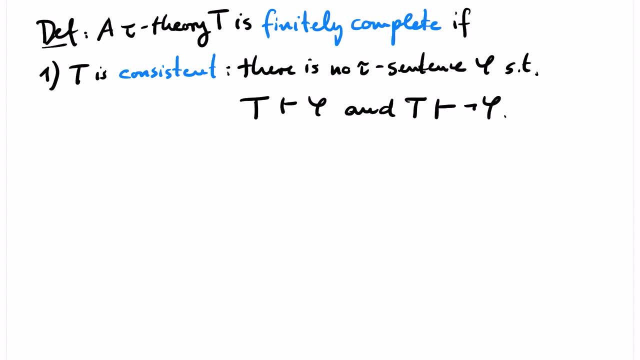 Of course, if you want to construct a model of t, this condition is certainly necessary. Second, for every tau sentence phi, either there is a formal proof of phi in t or there is a formal proof of not phi in t. Now, our lemma says that every finitely. 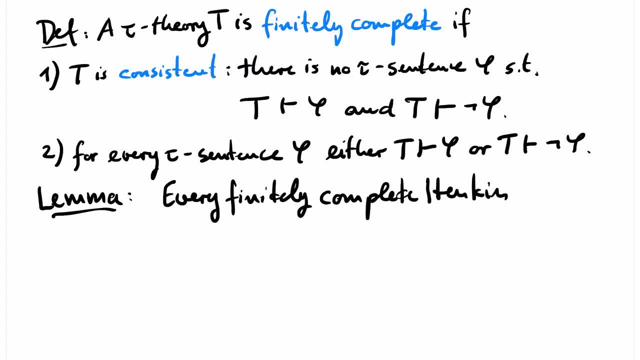 complete Henking theory has a model. The idea is that for such theories we can directly construct a model a by reading it off from the theory. Formally, the elements of our structure a are equivalence classes of Henking constants where c1 and c2 are equivalent. 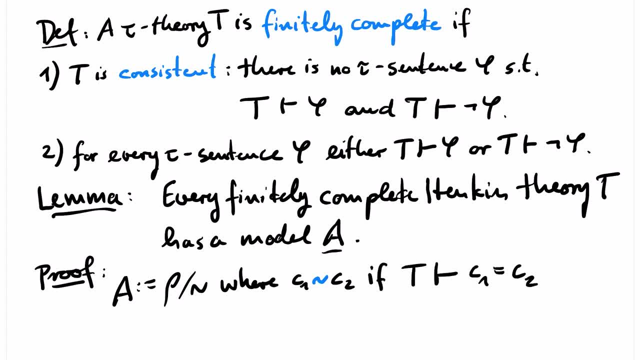 if there is a proof, a formal proof in c of c1 equals c2.. Note that this indeed gives an equivalence relation because of our axioms e1, e2 and e3.. We write c in square brackets for the equivalence class of c with respect to our 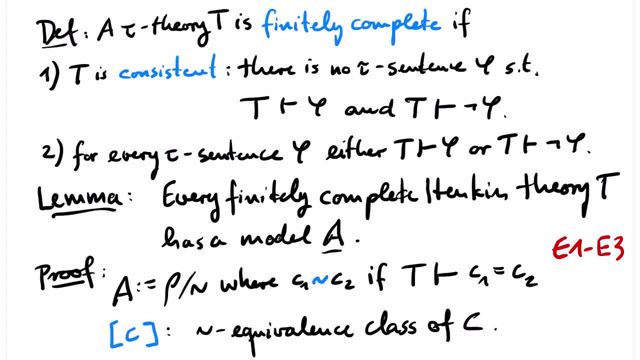 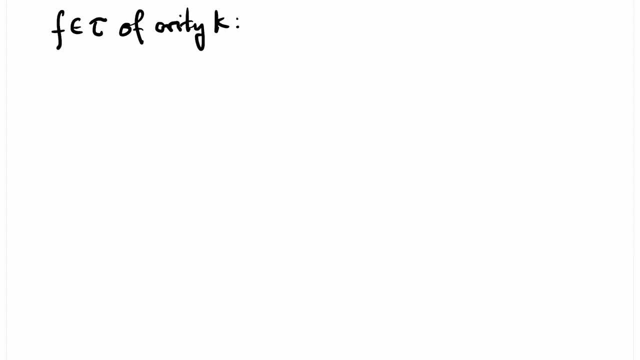 equivalence relation To construct our structure a, we also have to say how the operations and relations of a look like. If f is a function symbol of arity k in the signature tau, then the operation of a for f is defined as follows: It maps square, bracket c1. 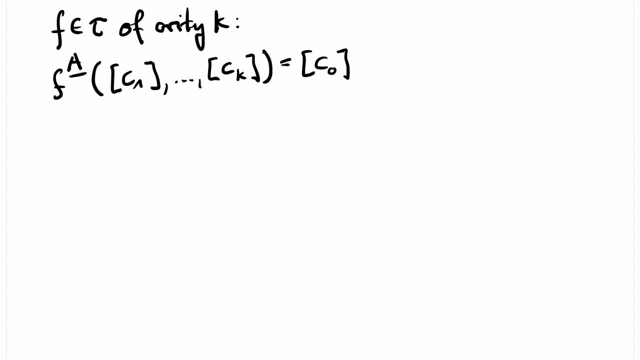 up to square bracket ck to square bracket c0. if there is a formal proof in t of the sentence f of c1 up to ck equals c0. It follows from the equality axiom e4 that this is well defined. One can also show that f is defined. 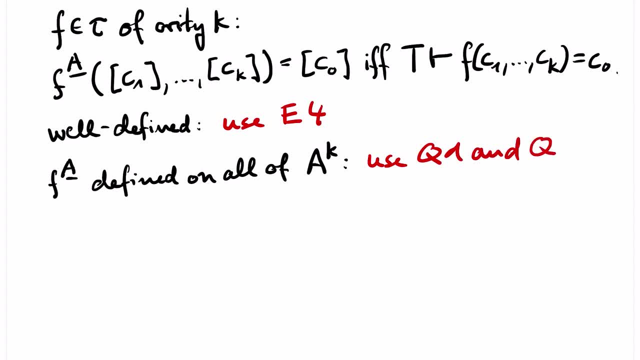 on all of a to the k using the axioms q1 and q3 and the assumption that t is a Henking theory. This is a bit technical and left to the reader. The relations of a are defined similarly and that's the entire construction. That's how a looks like. 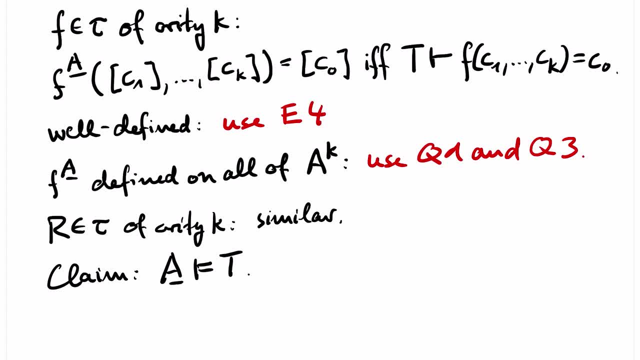 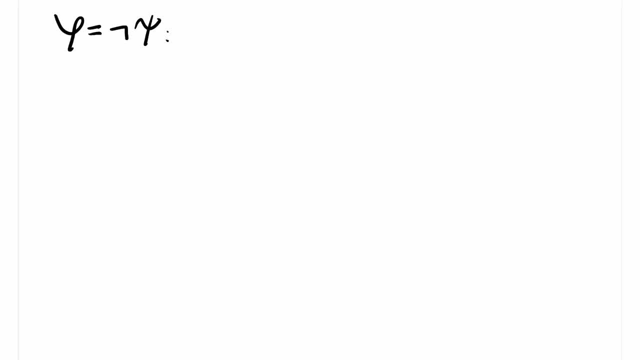 And we claim that a is indeed a model of t. Our proof is by induction on the size of sentences. If phi is of the form, not psi, then a models phi if, and only if, a does not model psi, If, and only if psi has no. 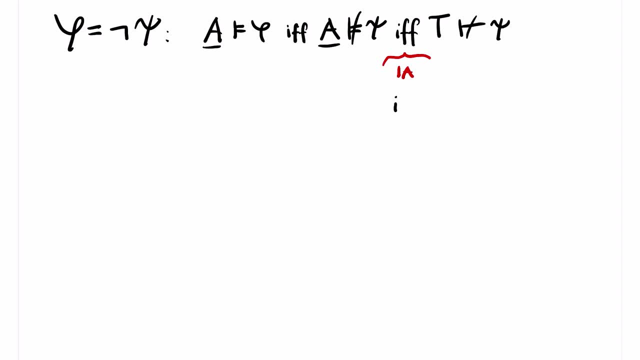 formal proof in t by inductive assumption. This in turn is the case if, and only if not, psi has a formal proof in t by finite completeness, And this is what we had to show If phi is of the form psi1 and psi2. 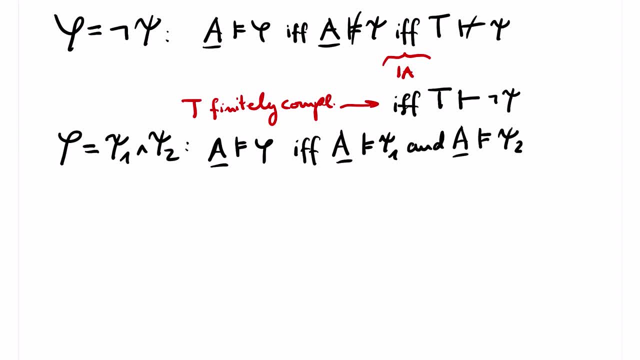 then a models psi1 and psi2, if, and only if, a models psi1 and a models psi2.. By inductive assumption, this is equivalent to psi1 having a formal proof in t and psi2 having a formal proof in t, And finally one can show that this is the case. 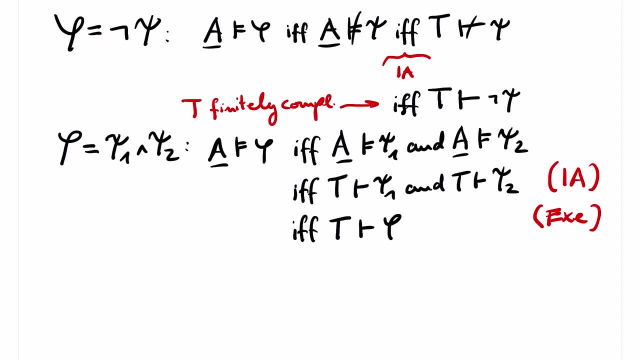 if, and only if, psi1 and psi2 has a formal proof in t. I leave this as an exercise. If phi is of the form exists x psi, then a models phi. if, and only if, a models psi of c for some hanking constant c by the construction. 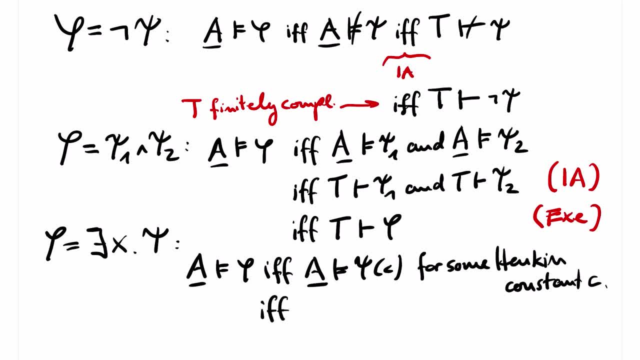 of a. This is the case if, and only if, phi of c has a formal proof in t by inductive assumption. And this in turn is the case if, and only if, phi has a formal proof in t. Here we have to use the axiom q3 and some. 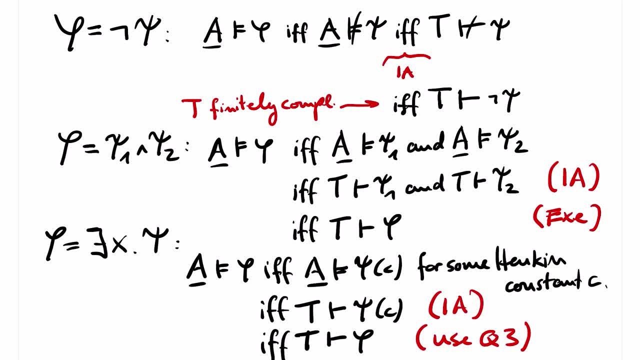 reasoning with formal proofs that I also leave to the reader, And this is the end of the proof. Interestingly, so far we have only used the axioms for equality q3, q1- also taught implicitly- and, of course, modus ponens, but not q2 and q4. 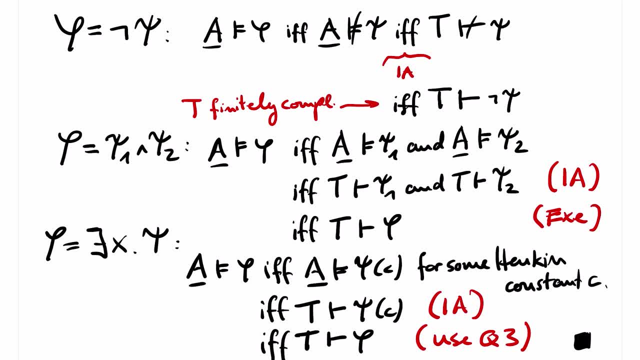 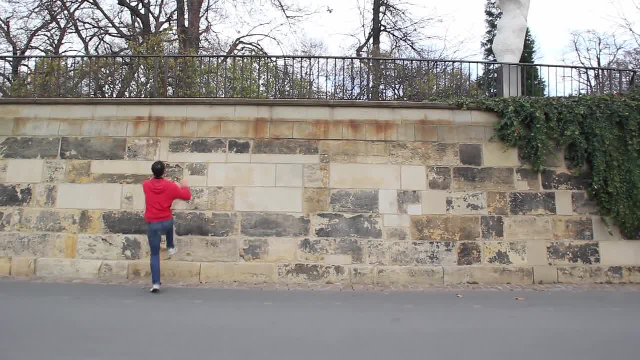 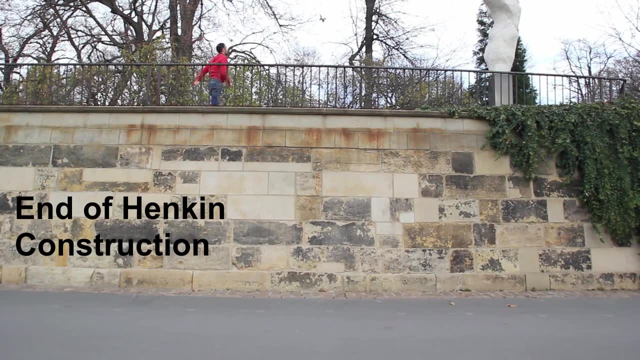 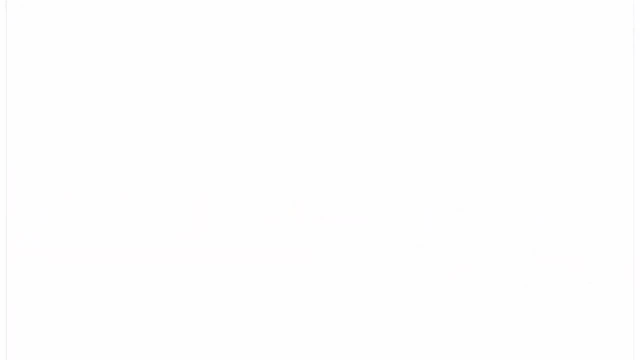 and q5.. They will be used later, Thank you, So all that is left for the proof of the completeness theorem is showing that if phi does not have a formal proof in t, then t union, not phi, can be extended to a finitely complete. 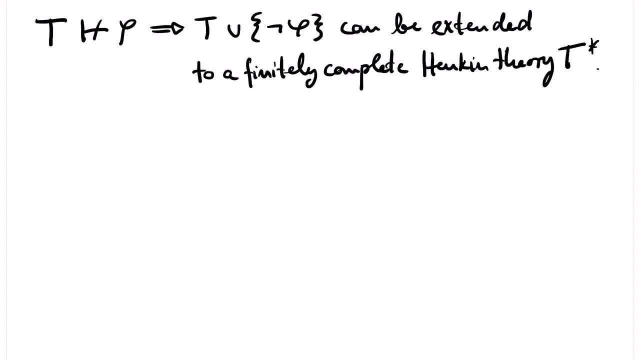 hankin theory, t star, because such a theory has a model and hence the reduct of this model to the original signature is a model of t union, not phi. First of all, if phi does not have a formal proof in t, then t union, not phi, is consistent. 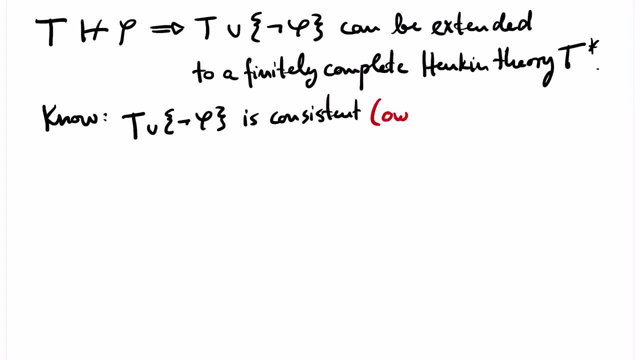 This requires proof, but you can find the full proof in the course notes. We now need new constant symbols for the hanking constants to define t star. They are defined as the union of an increasing sequence- rho zero, rho one and so on- of constant symbols, starting with the empty set. 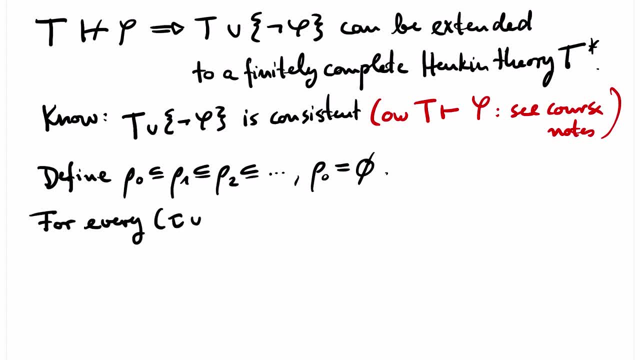 for rho zero. Now for every tau union, rho i, formula phi, with one free variable, f. we introduce a new constant symbol, c, phi, and define rho i plus one to be the extension of rho i by all those constant symbols. rho is then defined as the union of all. 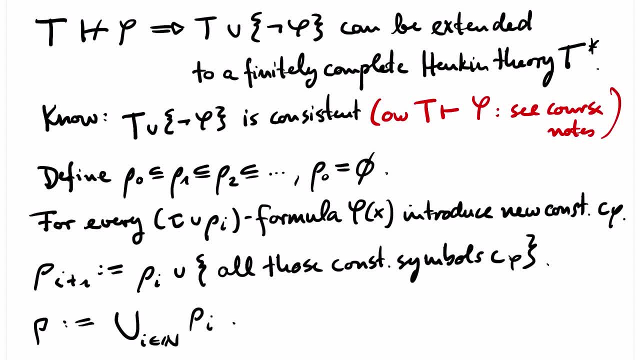 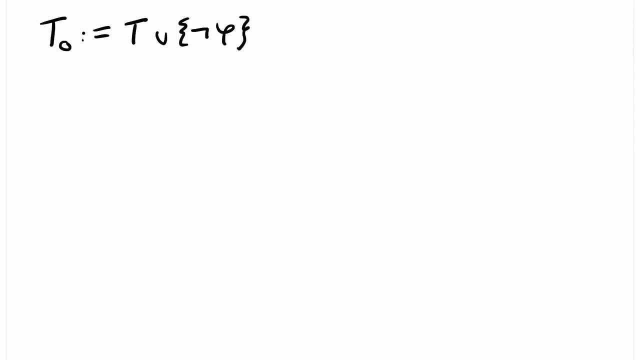 the rho i, and it is rho that will be the set of hanking constants for our theory t star. We define a sequence of theories t? i as follows: t zero is the set of t union, not phi. t i plus one is the union of t? i. 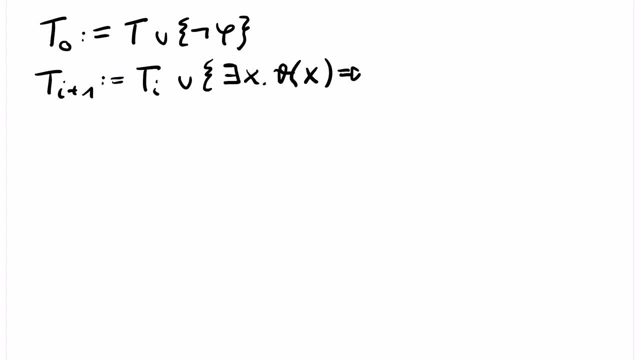 and the set of all sentences of the form. theta of x implies theta of c, of theta for all tau union rho i formulas theta. Our first claim is that t- i is consistent for every i and this can be shown by induction on i. It looks quite plausible. 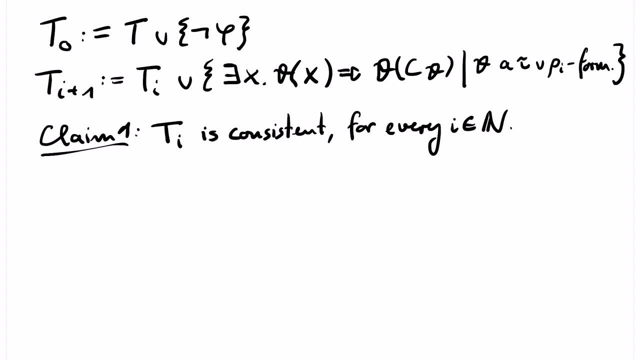 but to prove it in full detail takes some care. It is here where we use q2, q4 and q5. The next claim is that the union of all the t? i is consistent. This is actually quite easy to see, since every formal proof in a theory. 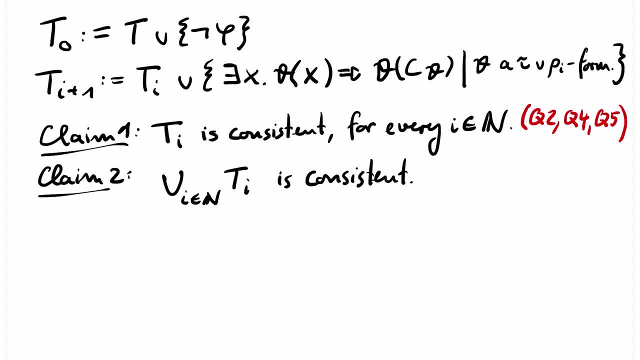 by definition, only uses finitely many sentences from that theory. So all of these sentences must come from the i for some sufficiently large i, and there we already know the statement. We can now apply Zorn's lemma and obtain a maximal with respect to inclusion consistent. 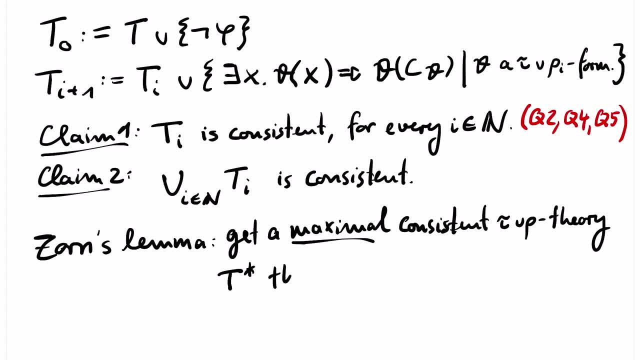 tau union rho theory. t star, which contains all the t, i and here we claim t star, is finitely complete and this follows for maximality. If a tau union rho sentence has no formal proof in t star, then t star together with the negation of that sentence.